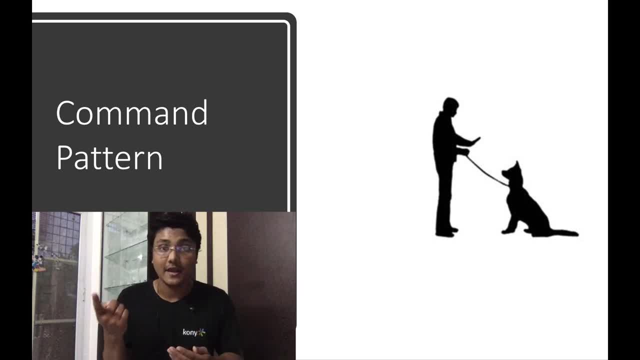 responsibility design pattern, which was the first pattern in the behavioral category. In this video we will be covering the command design pattern and I will be sticking to my old format. so we will first take a look at the definition for the command design pattern, Then we will take 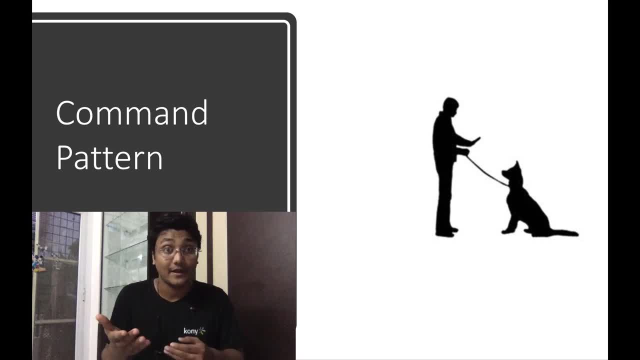 a look at the problems which arise, at how command design pattern comes to the rescue. Then we will take a look at the UML diagram for the command design pattern and at the end we will do some live coding to implement the command design pattern. So let's get started. So let's. 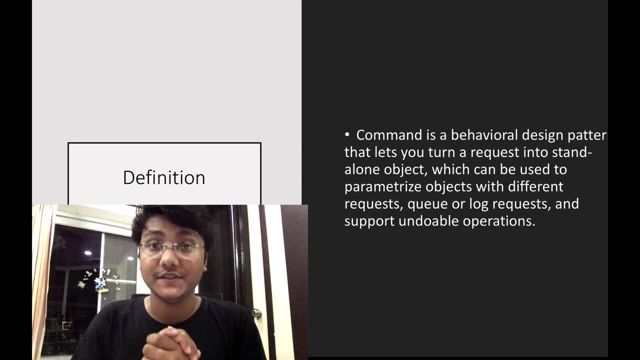 start by looking at the definition first. So command is a behavioral design pattern that lets you turn a request into a standalone object, which can be used to parameterize objects with different requests- queue or log request- and support undoable operations. so this is quite a lengthy definition with a lot of touch points. 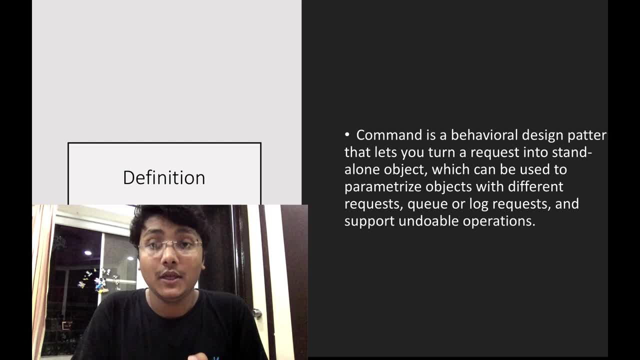 and which makes it difficult to understand for the beginners. so we will take this definition apart one by one and see what each part means and why is it important. so, before moving on to this definition, I will show you a simple use case scenario where you would like to implement the command design pattern. so 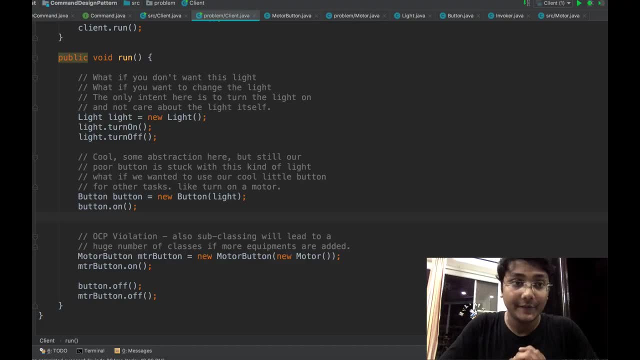 let's look at it so. this is our example here, and in this example, what we are trying to do is to switch on some light, switch it off and have a button to control that and also switch on some motors. so switching on a light is a request. is it's a type of request you want to handle, switching on a motor, or? 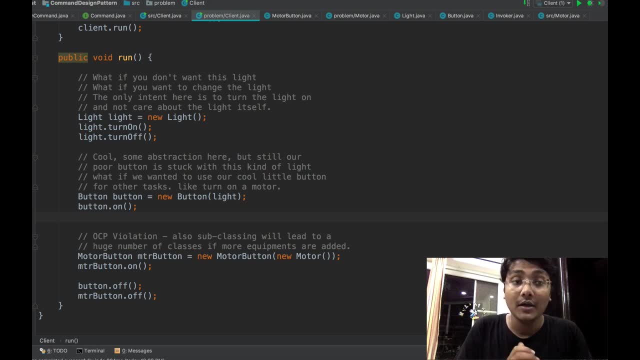 switching off a motor is also a type of requests which we want to handle. but there's a problem with this example. the problem is our code is tightly coupled to the receiver object. what we want to turn it on or off in first three lines. we are directly depending on the 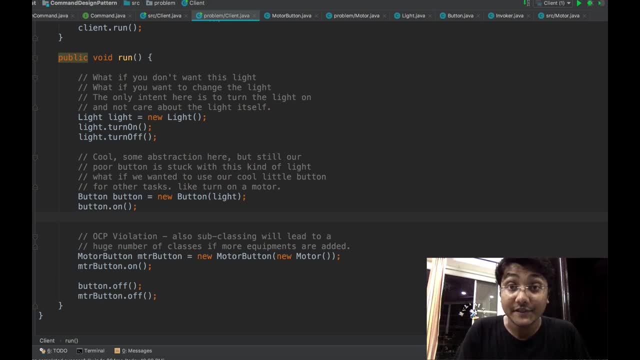 receiver object to turn itself on or off. so the problem with this is, let's say you don't want the same light you use you have used before. let's say you want to change the type of the light you are using, but since you are directly depending on the light class, you cannot change the methods. let's say the second. 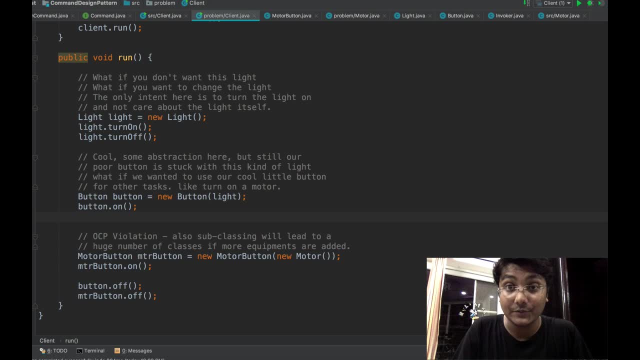 type of the light you're using is had a has some different minutes to turn it on or it has some different procedure to turn it on. the cold will pay right. instead of depending on the receiver directly, we should have abstraction to actually control behavior. we want to turn on the light for the receiver, but also not depend on the. 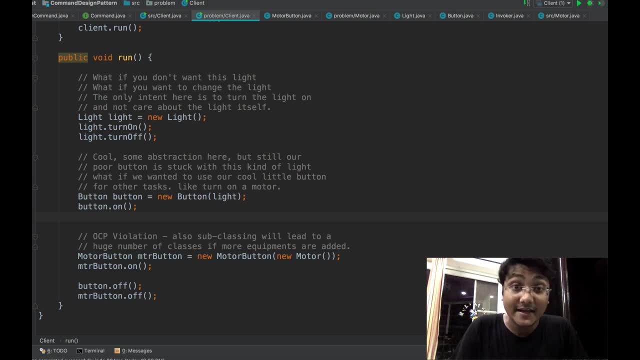 receiver directly, which will give us more flexibility. to enhance this further, what I did is added a button class which takes a light by a dependency injection and has an on method on it. the on method simply toggles the light on, which is good. we have added an abstraction for turning on the light, but the problem 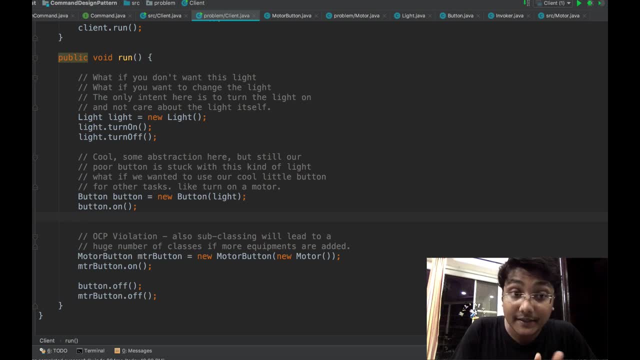 here is: our button is directly coupled to the light. now we cannot use this button class, which we can use to turn on anything except light, which is bad, because we don't want to directly couple our light with the button, because then the button will not be usable except with light. 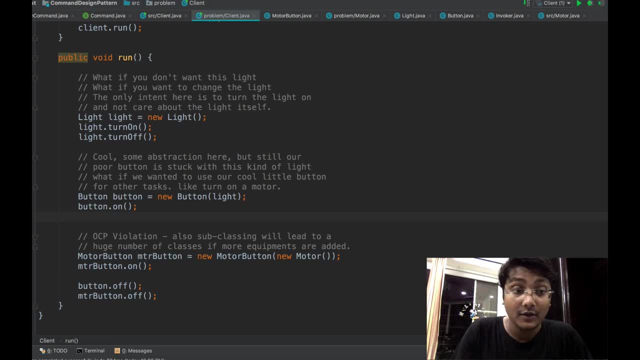 you. one more scenario is: let's say you want to add or turn on a motor with the same button, which is not possible because our button is directly coupled to light. so the most common solution which comes to people mind is to quickly go ahead and subclass this button, add a motor there and override all the methods and make it. 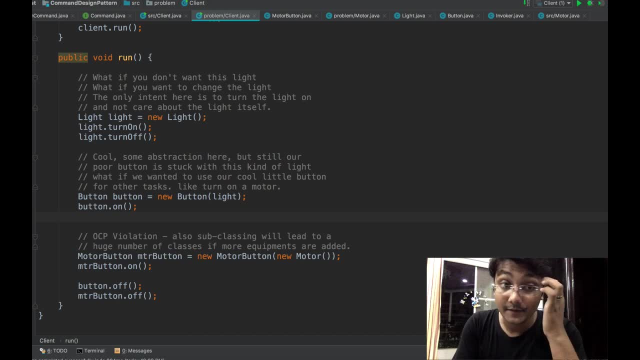 work. but the problem with this is, again, we are preferring subclassing over composition, which is bad. second is we are violating the open-closed principle, which says classes should be open for extension but closed for modification. but here we see that our class is not closed for modifications. so even if the behavior 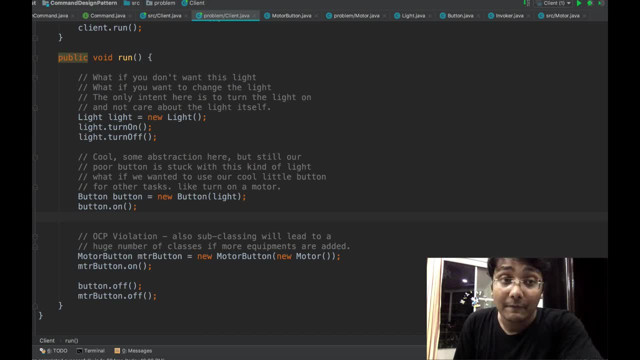 in the motor button changes, or let's say in the motor changes, our class will directly get affected. so let's have a look at the uml diagram for command pattern and see how command method tries to solve this problem. there is one more problem with this code, which is we cannot undo operations. there is no way. 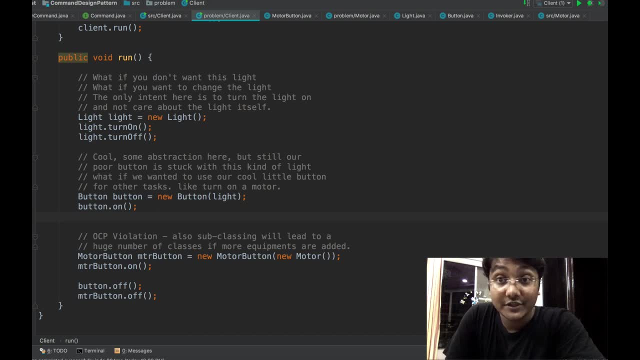 to track that, the order of the operations in which we perform them, and there's no way to undo it. so let's go ahead, take a look at the command design pattern, the UML diagram, and see how does it solves problem. so this is the UML. 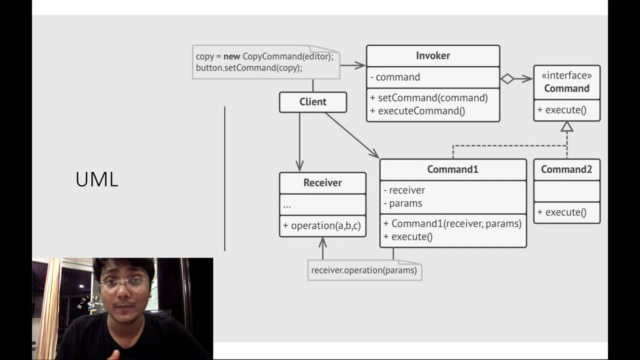 diagram for our command design pattern. in this UML diagram we have so many components, so let's look at them one by one. so the first component we have here is the client, which is the consumer of the requests. so this client will be sending requests to our invoker object. so invoker object is nothing but a proxy. 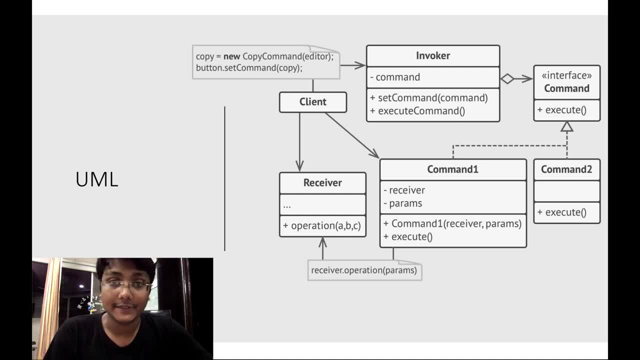 between our command interface and the client. so, using this invoker, we will be setting the command and asking the invoker to execute this command. now let's come to our next step. so let's come to our next step and let's go ahead and over command interface. our command interface has one method called execute. 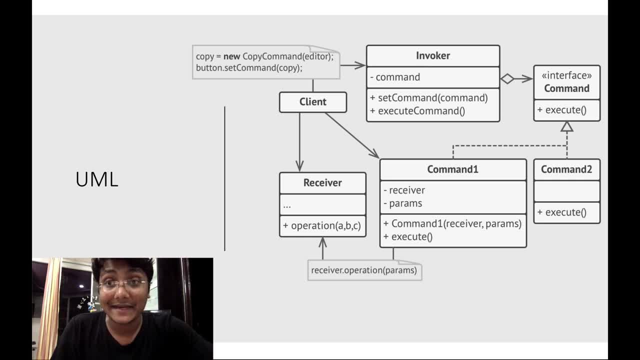 so this interface actually acts as the parent interface for all the tasks we want to do. so every command which wants to do something needs to provide its own implementation for the particular request. the request will also have a reference to a receiver. so in our case we have a command which will have a 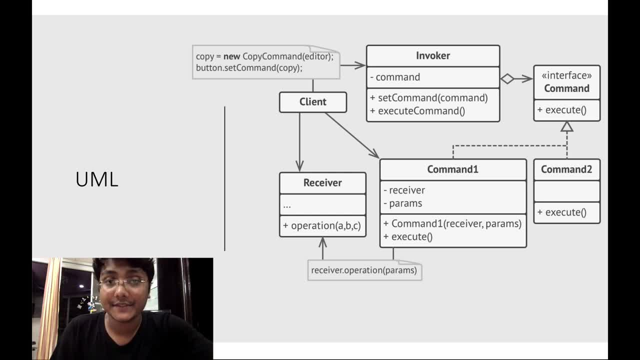 reference to a receiver which will actually process that request. so the the client will have a reference to an invoker and it will also set a command for the invoker to invoke. The invoker will in turn invoke the command by calling the execute method on the command. This execute method will call: 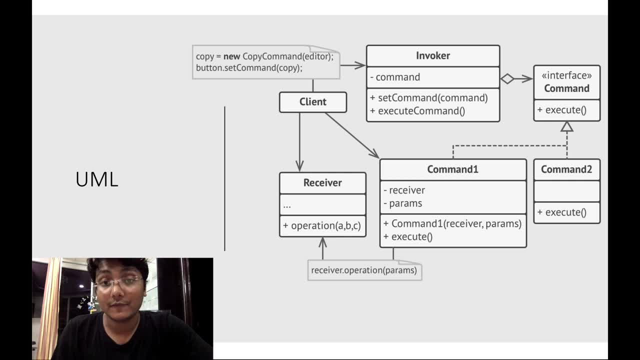 the reference receiver from the command object and perform the operation on it and return the result back to the client. So this is the general data flow diagram, or you can say UML diagram, for the command design pattern, and let's look this in action. So here in this coding example I have a one-to-one 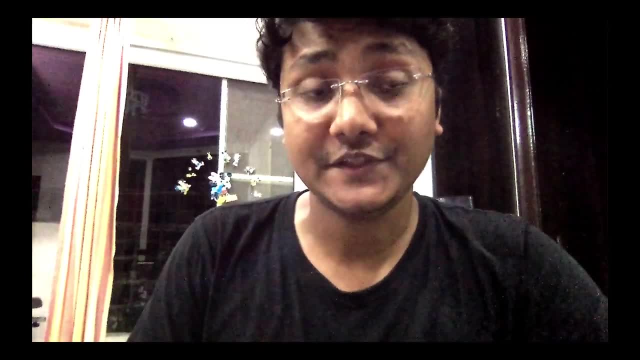 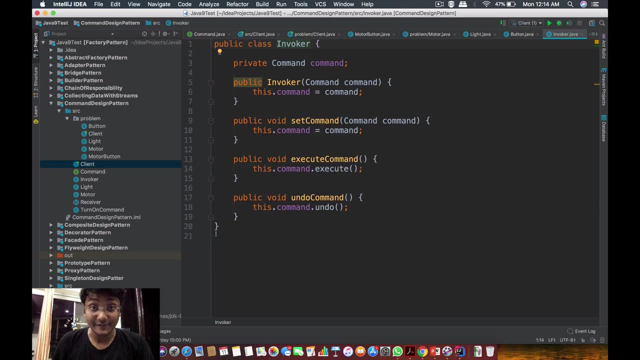 mapping the UML diagram. So the first thing which we saw in the UML diagram was our client class, and this client class has a reference to an invoker object. Let's go inside this invoker object and see what it does. So this: 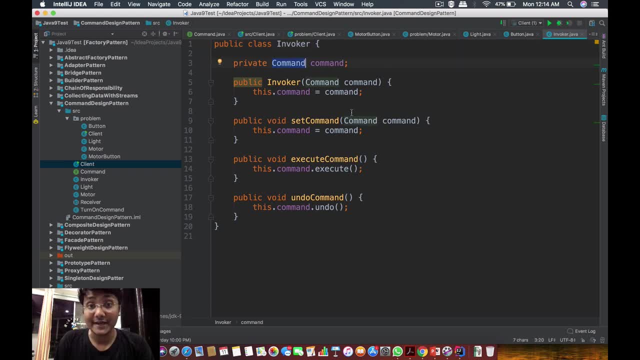 invoker object again has a reference to a command object and it has methods to set this command object and also install and instantiate this command using constructor injection. We have a method to execute this command and also undo this command. So let's quickly go inside. 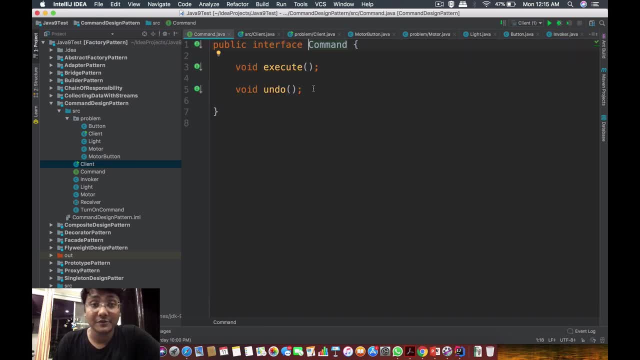 this command object. So this command is basically an interface which provides two methods, which is execute and undo. So I have added this one more method called the undo method, so that I can show you how can you keep track of the commands and also reverse the operation you perform with this command design pattern. 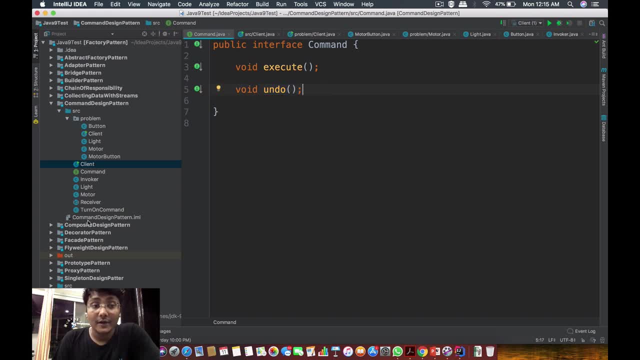 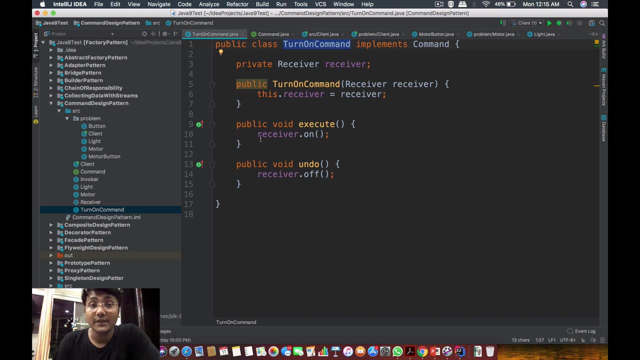 So I have created one command which is called the turn on command, and this turn on command implements this command. so it has to provide implementations for the execute method and the undo method. So basically, this turn on command gets a receiver and what it does is it turns the receiver on or either off, So it basically signals: 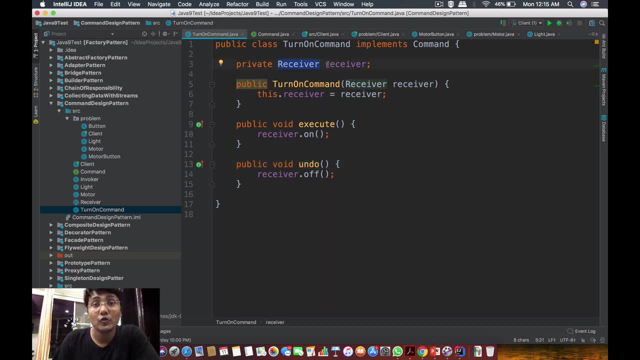 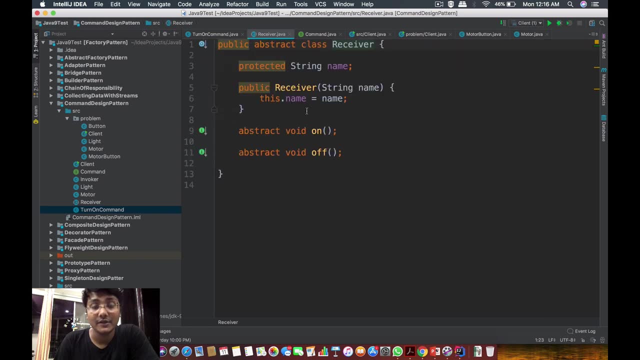 the receiver to be turned on or turned off. and the receiver could be anything. It could be a light bulb, it could be a motor, it could be anything which can be turned on or off. So let's go to the receiver class. So we see that a receiver 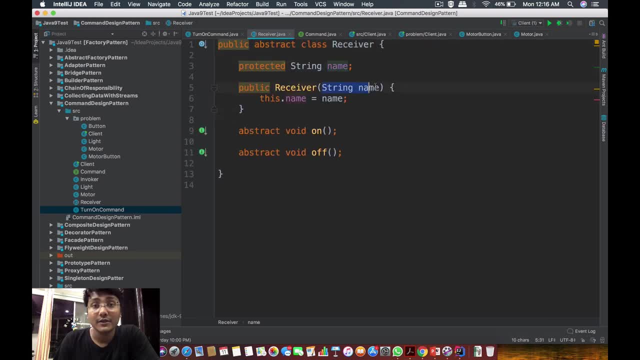 is an abstract class which has a name which we can set via constructor, and it has two abstract methods, which is on and off. So, since this is an abstract class, we need to provide the implementation using the subclass for this on and off method. So let's go to. 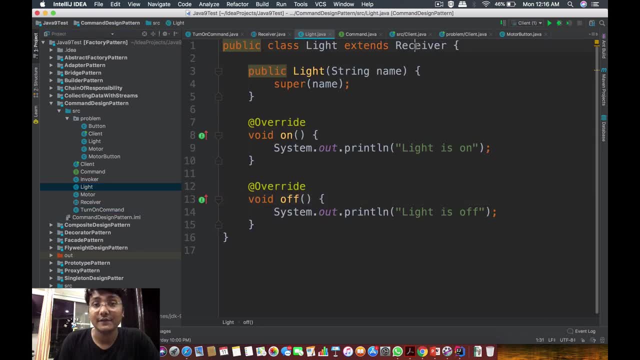 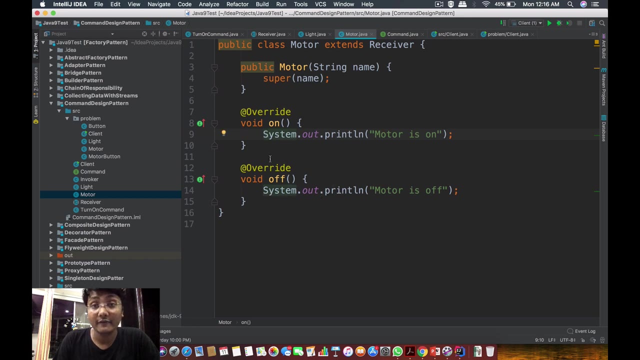 our light class, which is again a receiver, and it provides the implementation for the on and the off method. Similarly, we have our motor class, which is also a receiver, and it also provides the implementation for the on and off off method. so, whatever is a receiver, it can be turned on or it can be turned off. so let's go to 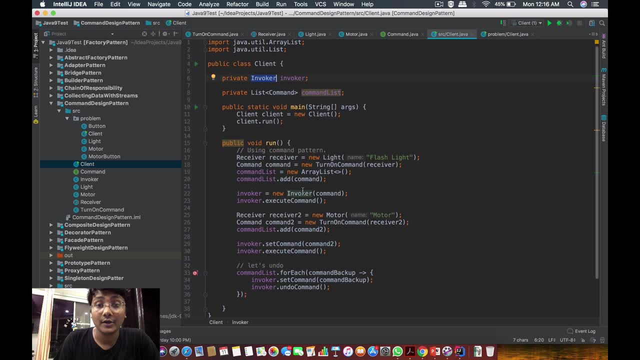 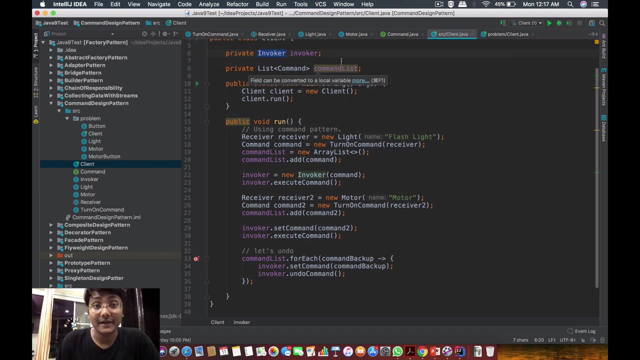 our client command and see how flexible is it to actually create and dispatch requests to the to these command objects and let the invoker take care of invoking them. so this is our client class. it has a reference to the invoker and also maintains a list of command. so this is the 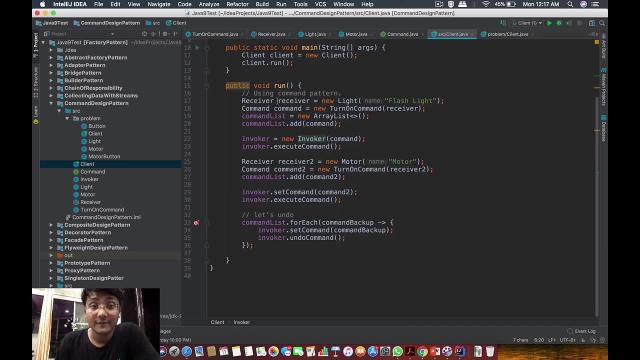 method which is being called when we execute this program, so the receiver. we are creating some receivers here for now. so our first receiver is a light object which is a flashlight, and our first command is the turn on command. so this turn on command takes a receiver because we want to. 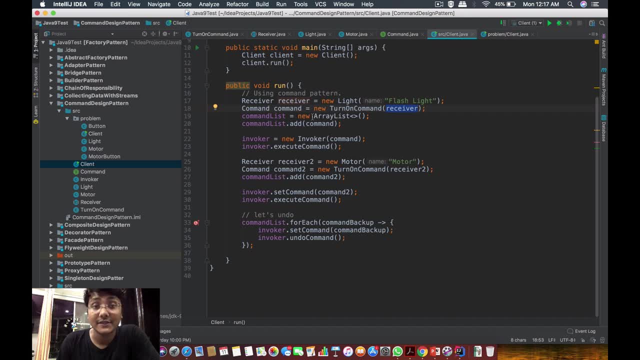 turn it on. so, before turning it on, what we are doing is actually pushing this command to our command list back. so after pushing the list, what we are doing is we are creating the invoker, we are instantiating the invoker with this command and we are asking the invoker to actually execute. 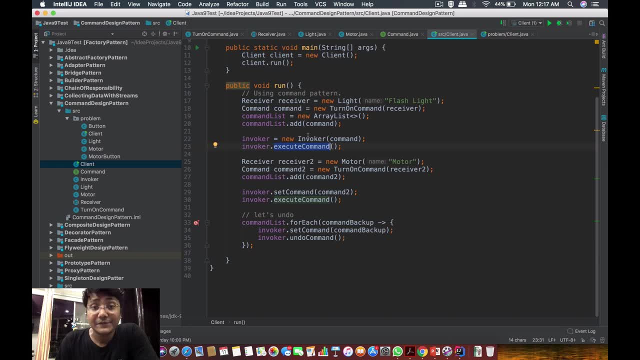 this command for us. after the execution, we are creating the second receiver, which is called the motor, and we are also creating a new command to actually turn on this motor. so, after creating the second command, we are also adding it to the command list, and then what we are doing is setting. 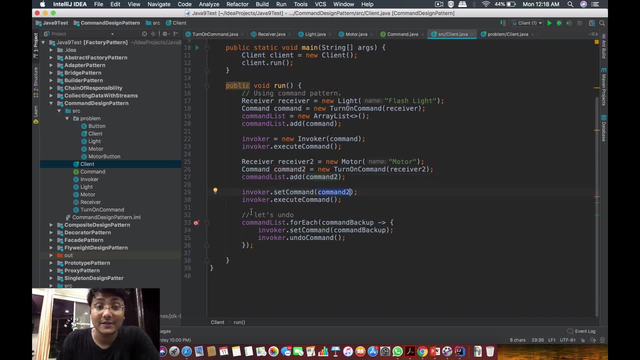 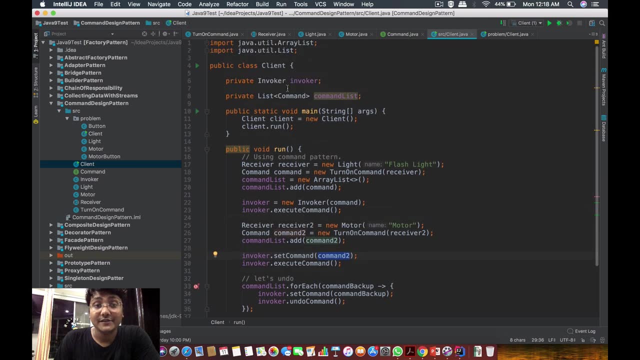 the command 2 for the main command for the invoker, so that we- this invoker- can execute the command 2 and turn on the motor. now, after executing this command, since we have the history of the commands in this list- command list- what we can do is iterate on this list and call the undo method for each command. so 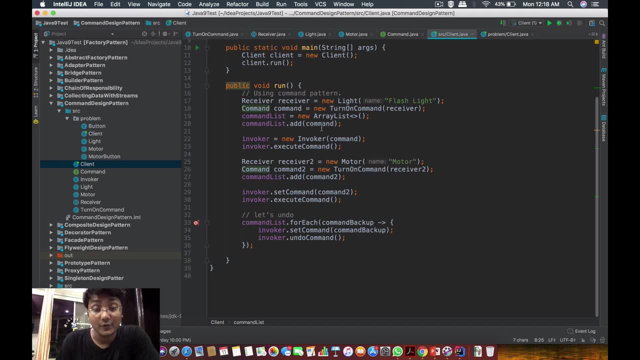 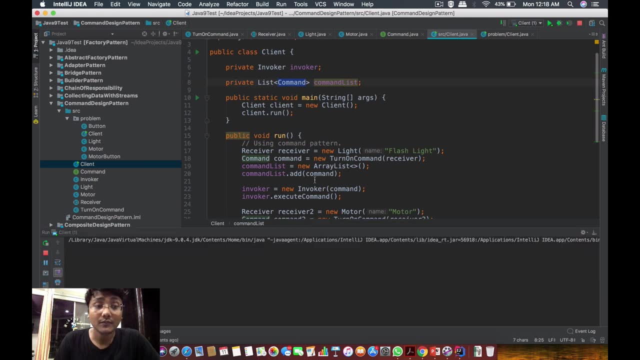 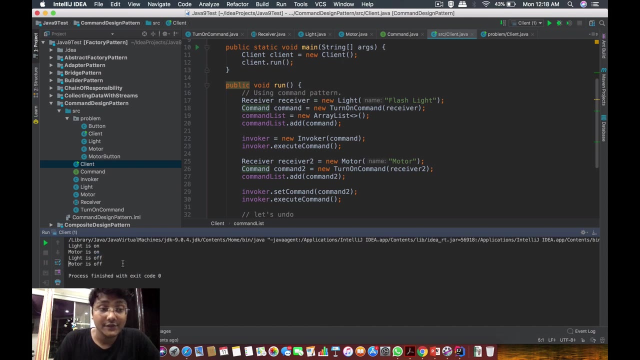 whatever this command does, we can actually reverse the operation for each command in the command list. so let's run this code and see this in action. so, after running this code, what we get as output is: light is on, motor is on, light is off and motor is off. since you see that, whatever is the order of the command, 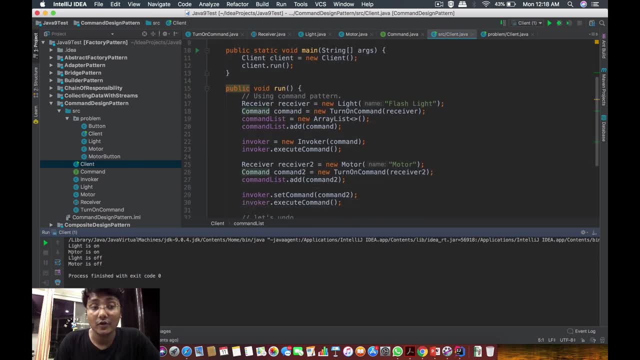 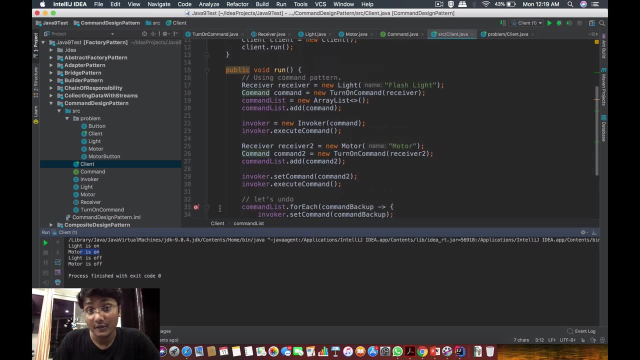 this same order is maintained. so first we did the light on command, then we turned on the motor, then, in the same order, we did the undo operation for each command. now see, you see how flexible is it to add multiple commands to your command list. keep a track of all the commands, all the request. 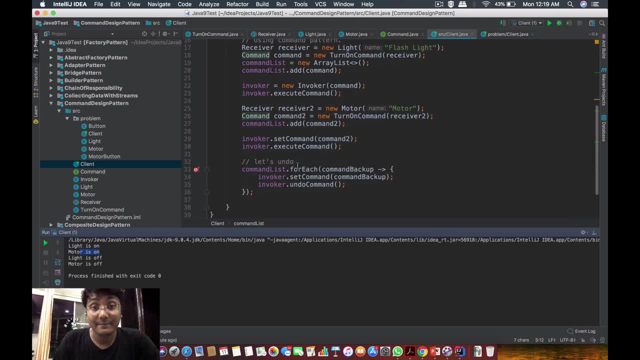 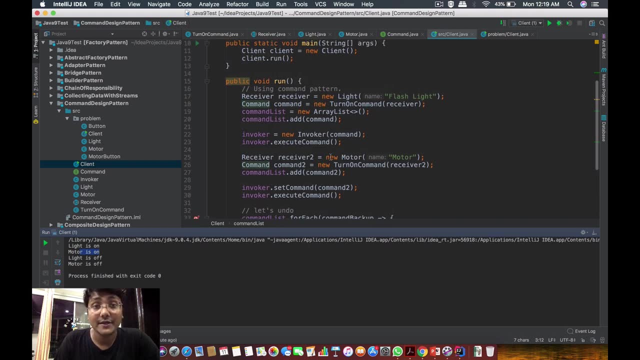 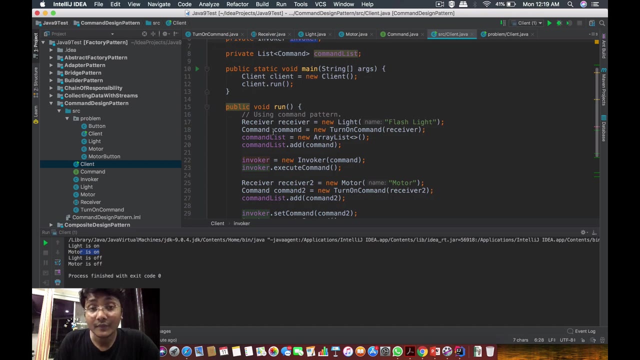 object what you are going to perform, and also keep it separate and independent from your client code. so your client code basically knows nothing about this command object, it only knows about the invoker and the invoker invokes all these commands. so here i have, uh, created all these commands here. 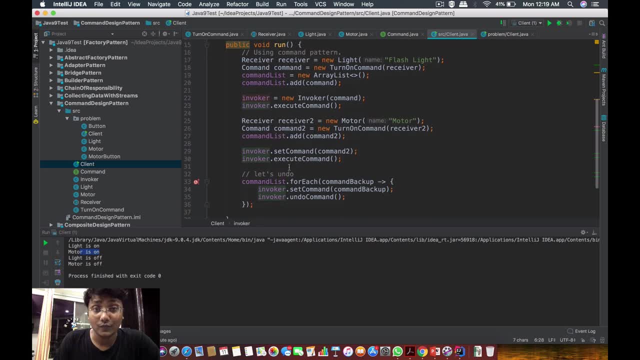 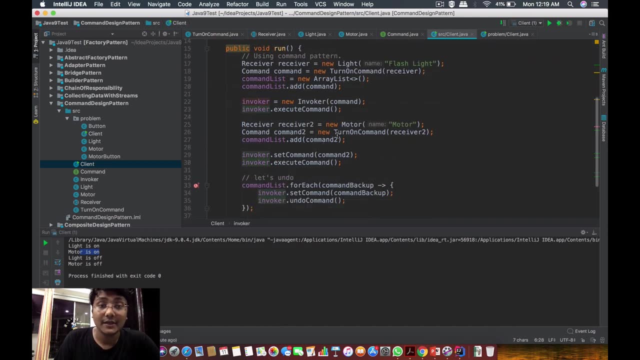 objects in this client only. but in the actual scenario, what you will be doing is, uh, injecting these command objects dynamically in the invoker using dependency injection and see how beautiful is it to resolve all those dependencies at runtime. okay, so thank you, guys, for sticking up with me for 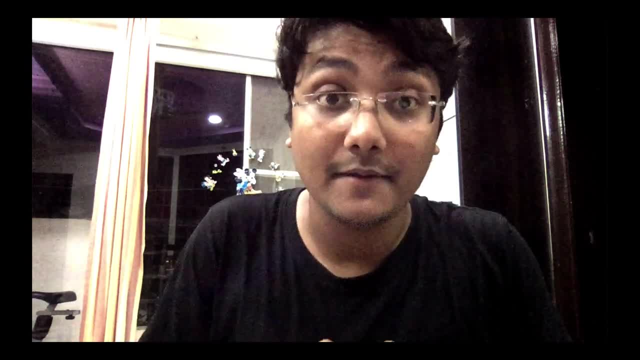 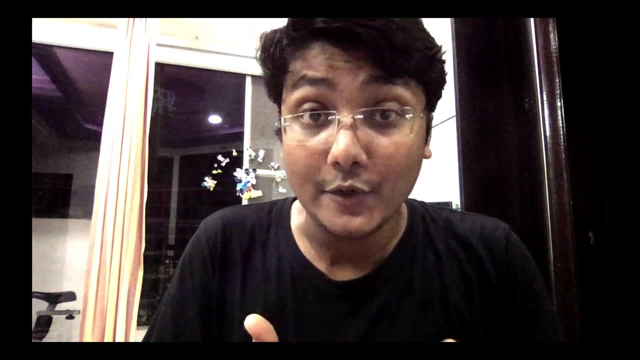 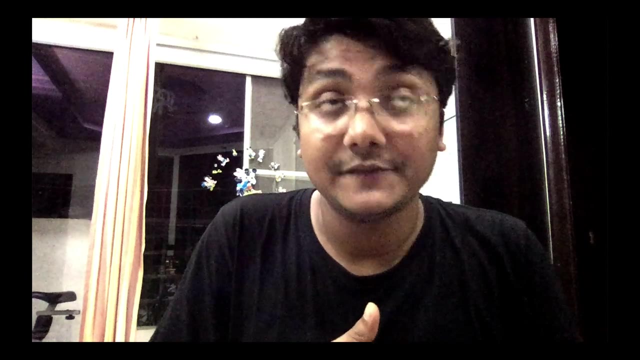 so long. it's around 12 minutes. i hope you have understood the command design pattern, so the main intent behind this command design pattern: if you want to encapsulate the request object and you want to do undoable operations and keep track of all the requests your system is processing, then you should definitely check out this command pattern.